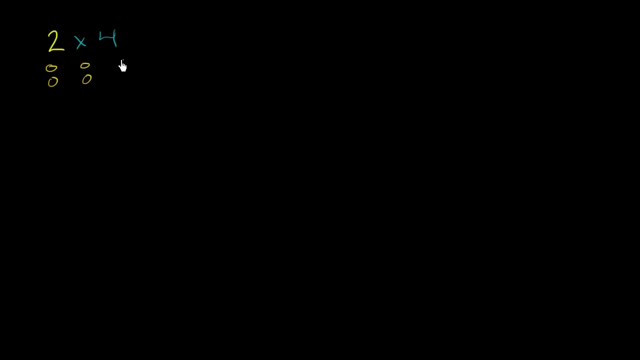 So that is one group of two, two groups of two, three groups of two and four groups of two, And we learned many, many videos ago that this, of course, is going to be equal to eight. But we could express a very similar idea with division. 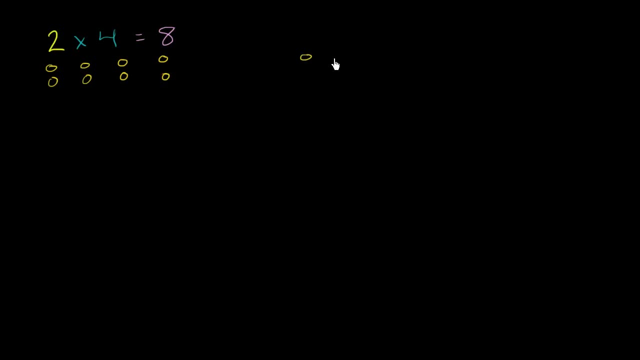 We could start with eight things. So let's start with one, two, three, four, five, six, seven, eight things. So now we're going to start with the eight And we could say: well, let's try to divide that into four groups, four equal groups. 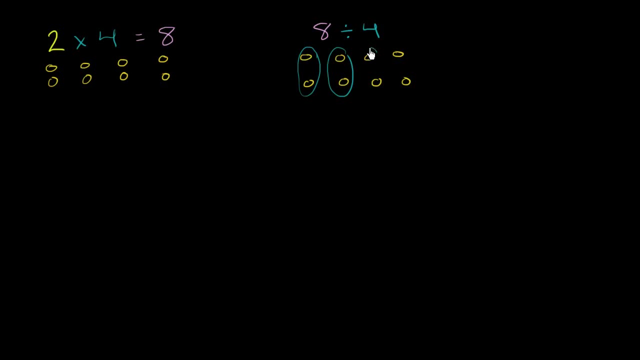 Well, that's one equal group, two equal groups, three equal groups and four equal groups. And we see, when we start with eight, divide it into four equal groups. each group is going to have two objects in it. So you probably see the relationship. 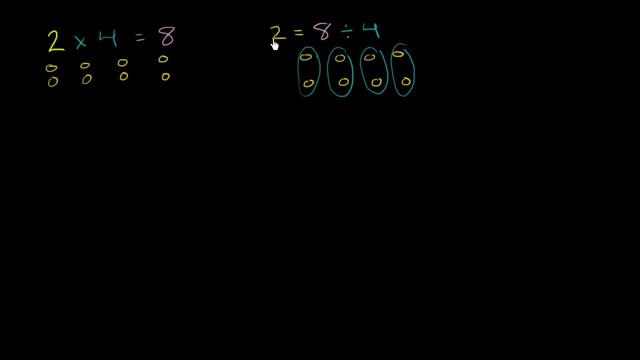 Two times four is eight. Eight divided by four is two, And actually if we did eight divided by two, we would get four, And this is generally true. If I have something times, something else is equal to whatever the product is. if you take the product, 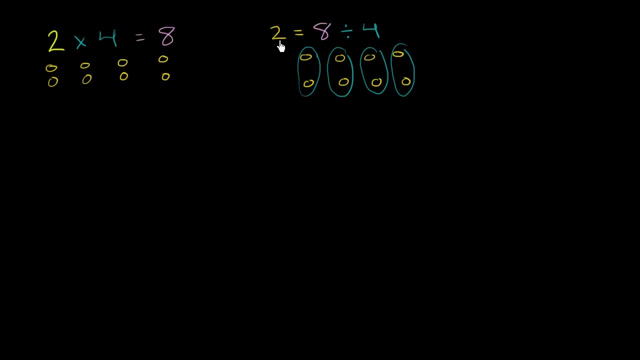 and divide by one of those two numbers, you will get the other one, And that idea applies. It applies to fractions And it actually makes a lot of sense with fractions. So, for example, let's say that we started off with 1 third. 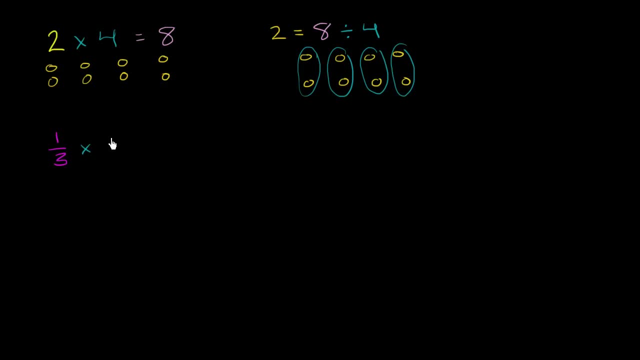 And we wanted to multiply that times three. Multiply by three. Well, there's a couple of ways we could visualize it. Actually, let me just draw a diagram here. So let's say that this block represents a hole And let me shade in 1 third of it. 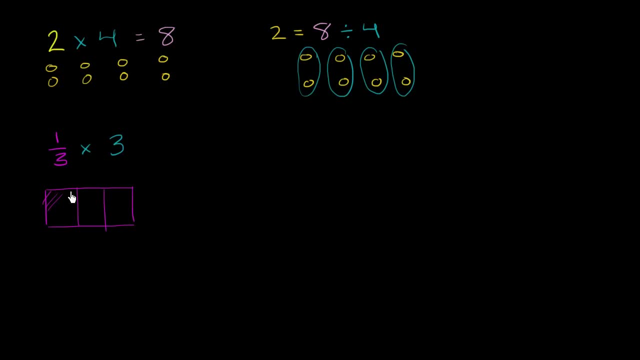 Let me shade in 1 third of it, So that's 1 third. We're going to multiply by three, So we're going to have three of these 1 thirds. Or another way of thinking about it is going to be 1 third plus. 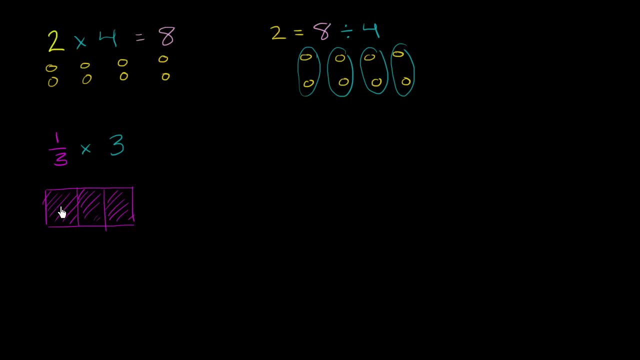 another 1 third plus another 1 third. That's our first third, our second third and our third third And we get the whole. This is 3 thirds or 1.. So this is going to be equal to 1.. 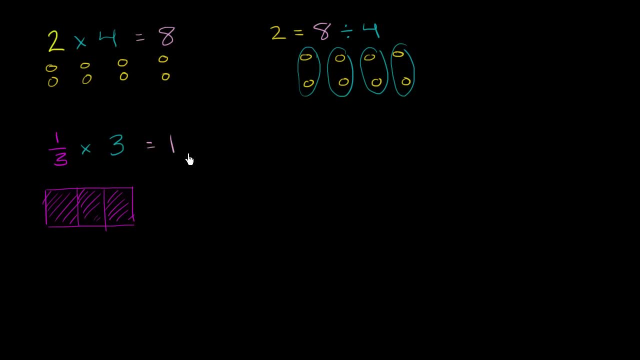 So you use the exact same idea If 1 third is equal to 1.. If 1 third times 3 is equal to 1, then that means that 1 divided by 3 must be equal to 1 third. And this comes straight out of how we first. 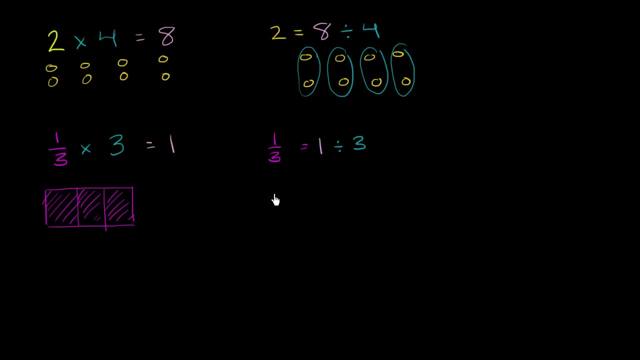 even thought about fractions. The first way that we ever thought about fractions was: well, let's start with a hole, And that hole would be our 1. And let's divide it into three equal sections, the same way that we divided this 8 into four equal groups. 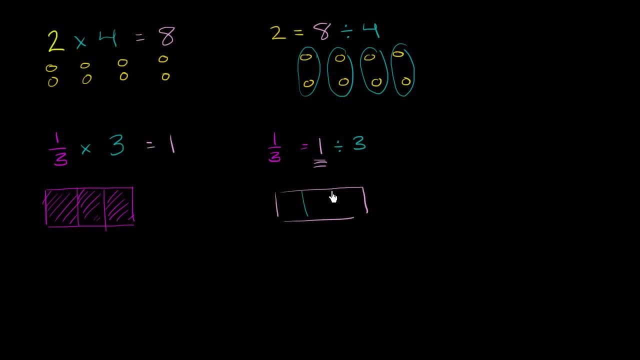 So if you divide this into three equal sections, the size of each of those sections is going to be exactly 1 third. Now this leads to an interesting question that might be popping in your brain. Notice: we have 1 as a numerator, 3 as a denominator. 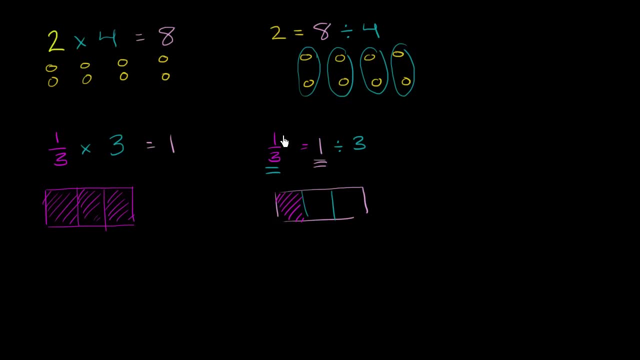 And we just said that this is equal to the numerator divided by the denominator. 1 over 3 is the same thing as 1 divided by 3.. Is this always true For a fraction? Well, let's just do the same thought experiment. 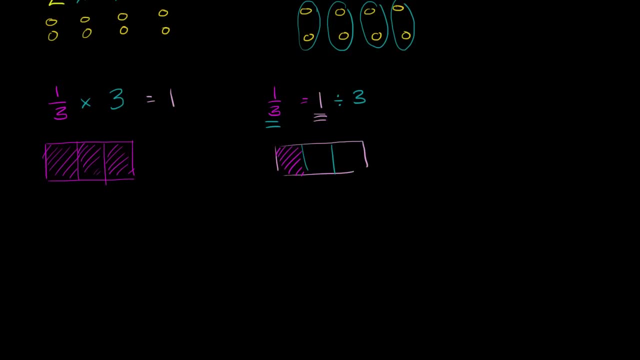 but let's do it with a different fraction. Let's take 3 fourths and multiply it by 4.. So, multiply it by 4.. So once again, let's see if I could draw a fourth here. Let me do this in a new color. 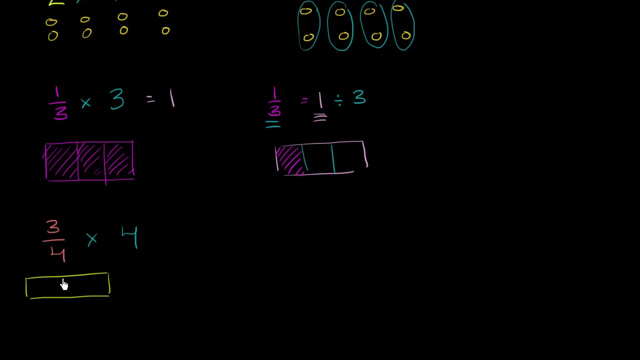 So let's say that this block right over here is a hole. I'm going to divide it into four equal sections. So now I've divided it into fourths And let me copy and paste it so I can use it multiple times. So copy. 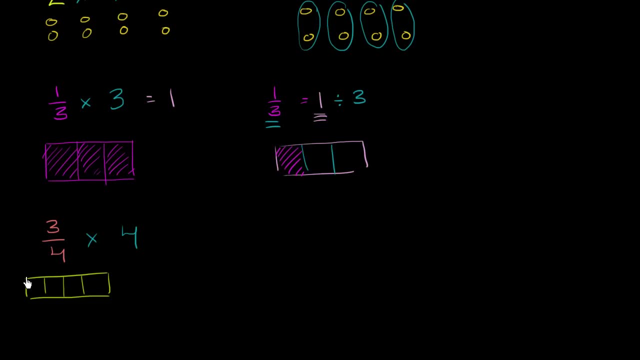 All right Now 3 fourths, that's going to be 1.. We can assume I didn't draw it perfectly. Actually, I could draw it a little bit better than that- just to make the four equal sections actually look equal. So that looks like a little bit better of a job. 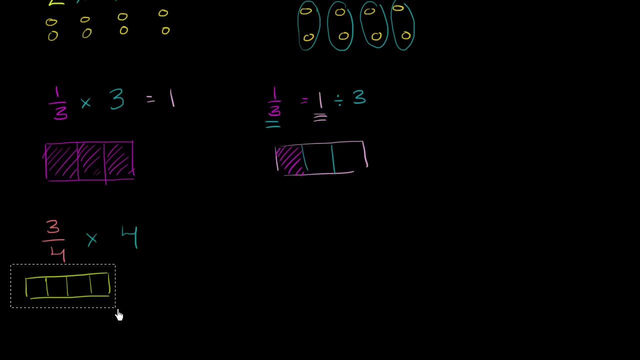 I'm trying to make them four equal sections And let me copy that one, So let me use it for later. Now, 3 fourths: this is four equal sections, And 3 fourths represents three of them: 1,, 2, 3.. 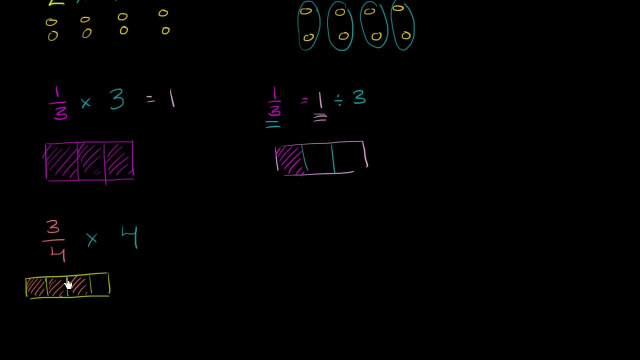 But now we're going to multiply it by 4. So we're going to have 3 fourths four times. So we're going to need some more holes here, So let's throw in another hole. So this is one 3 fourth. 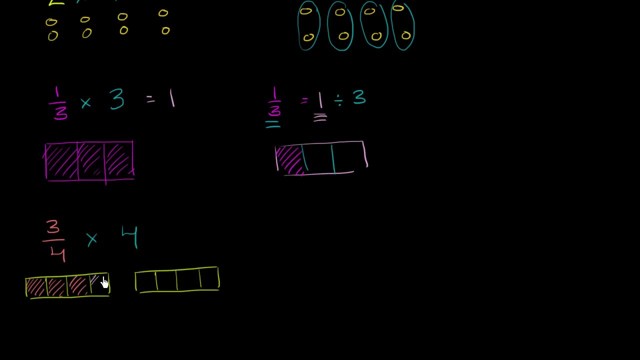 Now let me do the next 3 fourth in another color. So this is another, That's a fourth, That's a second fourth, That's a third fourth, That's another 3 fourths. And now let's do so. we've done two, 3 fourths just now. 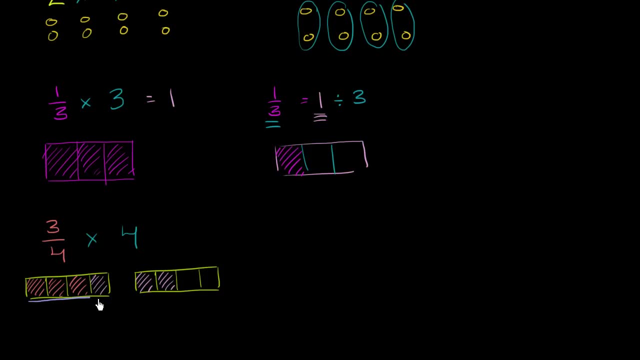 Let me make it clear: This is the first 3 fourths, And then this plus this is the second 3 fourths. Now let's do a third 3 fourths And we're going to have to use another hole right over here. 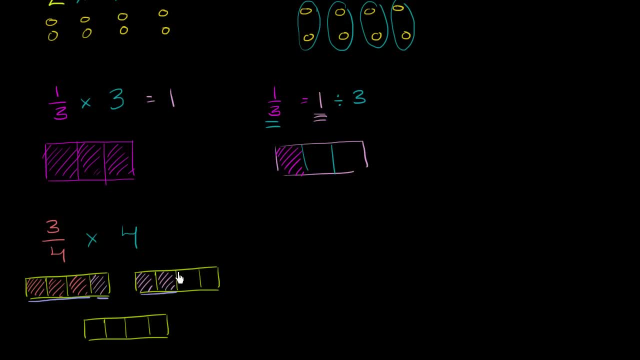 And I will do that in this color. So my third, 3 fourths. So here's a fourth. Here's my second fourth. Here's a third fourth. So in green, I have another 3 fourths, And now we need four, 3 fourths. 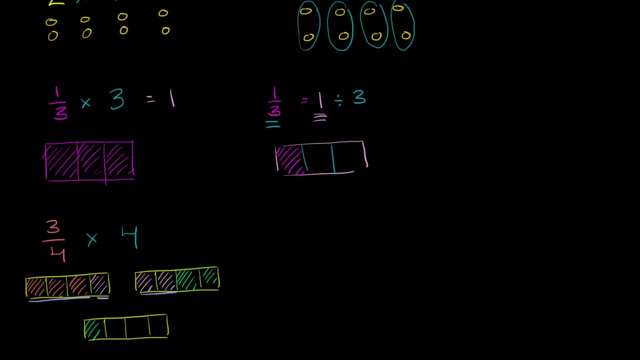 So let's do that In a color I have not used yet, maybe white. So that's a fourth, That's 2 fourths And that is 3 fourths. So notice now I have 1, 3 fourths, 2, 3 fourths, 3, 3. 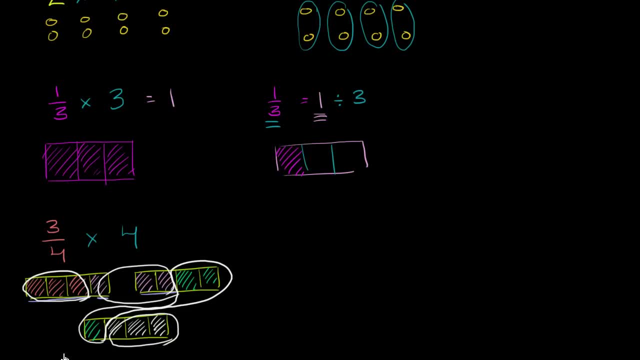 fourths and 4: 3 fourths. And what did I do when I got those 4: 3 fourths? Well, it's pretty clear. This is turned into 3 holes, So this is equal to 3 holes. 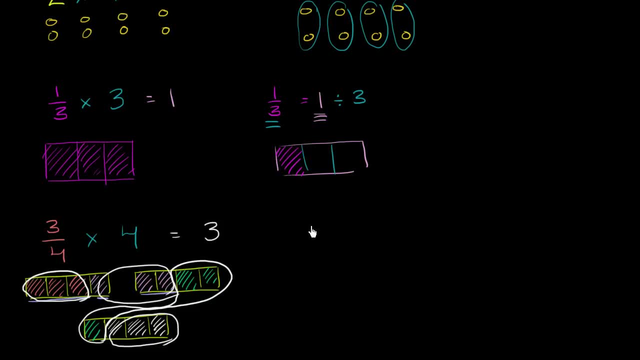 Well, if 3 fourths times 4 is equal to 3, that means that 3 divided by 4 is equal to 3 fourths. So the same idea again: 3 over 4 is the same thing as 3 divided by 4.. 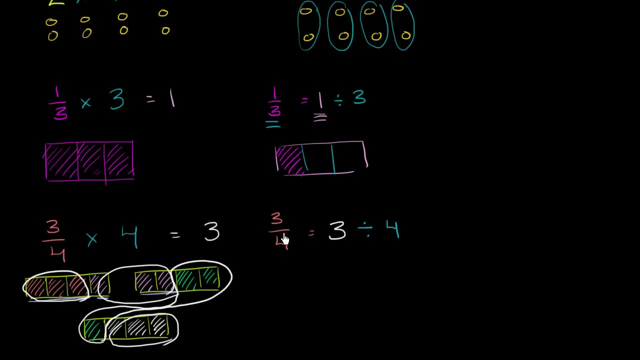 And in general this is true. The fraction symbol here can be interpreted as division And looking at this diagram right here, it made complete sense. If you started with 3 holes and you want to divide it into 4 equal groups, 1 group, 2 groups, 3. 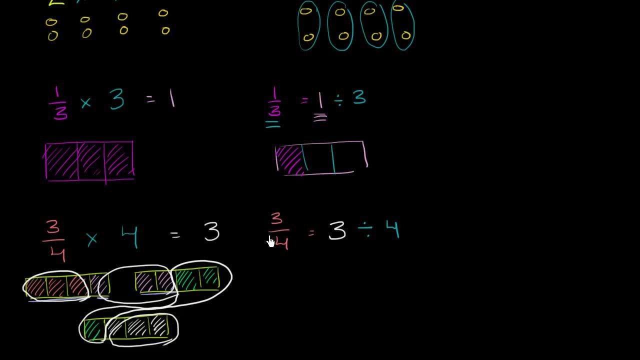 groups: 4 groups. each group is going to have 3 fourths in it.